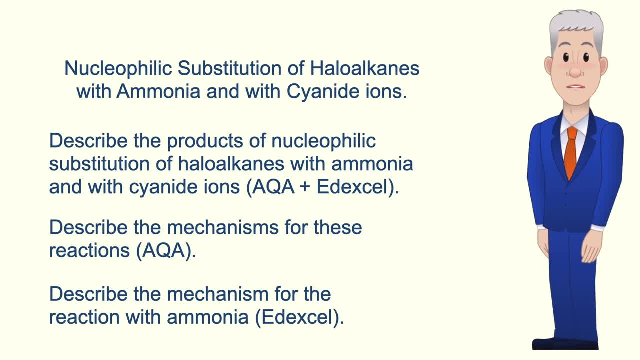 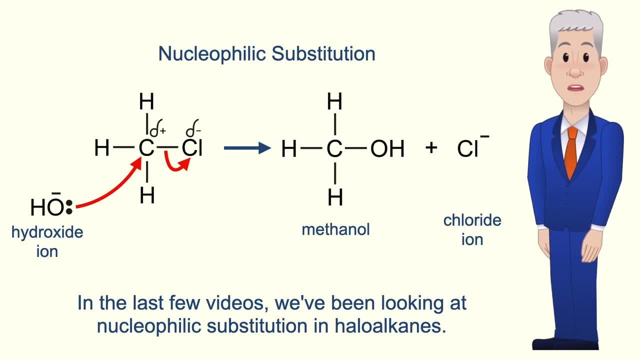 to be able to describe the mechanisms for these reactions, And if you're following the Edexcel spec, then you need to be able to describe the mechanism for the reaction with ammonia. only In the last few videos we've been looking at nucleophilic substitution in haloalkanes. 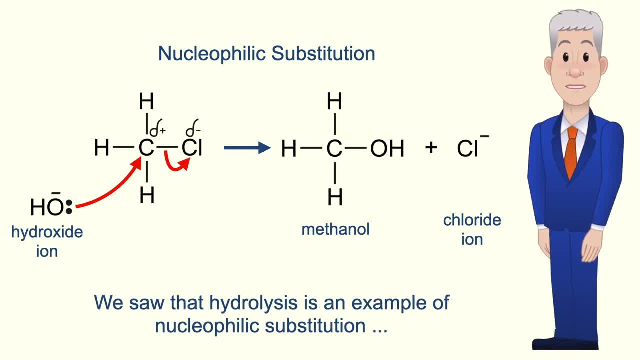 We saw that hydrolysis is an example of nucleophilic substitution, with the hydroxide ion acting as a nucleophile, And if you haven't seen that video, then I'd recommend that you watch it. In this video we're looking at the nucleophile's: ammonia and the cyanide ion. Let's start with. 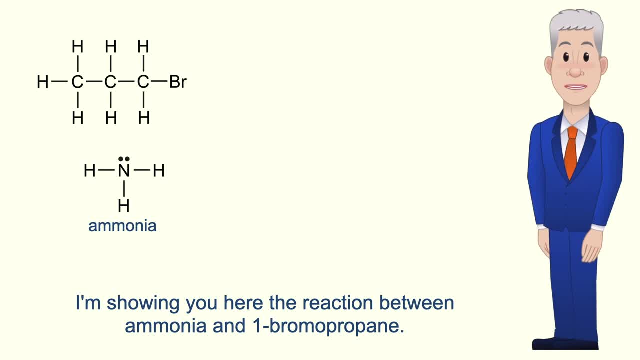 ammonia. I'm showing you here the reaction between ammonia and 1-bromopropane. This reaction is a reaction between ammonia and 1-bromopropane. This reaction is a reaction between ammonia and 1-bromopropane. This reaction takes place in two stages. In ammonia, the nitrogen atom. 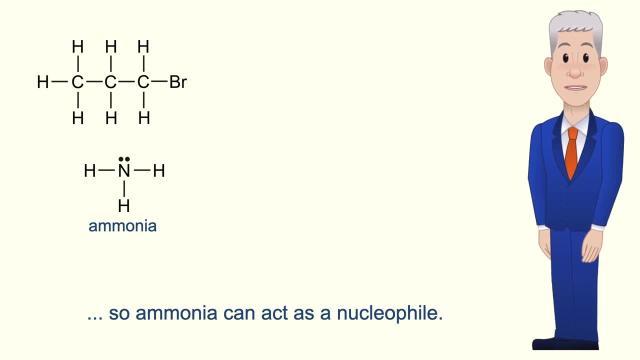 has a lone pair of electrons, so ammonia can act as a nucleophile. The lone pair of electrons on the nitrogen atom is attracted to the positively charged carbon atom in the haloalkane. The nitrogen atom donates the lone pair of electrons to form a covalent bond to the carbon atom, Now a carbon. 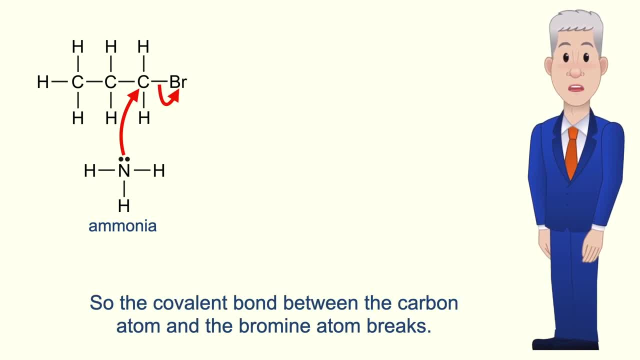 atom can have a maximum of four bonds, so the covalent bond between the carbon atom and the bromine atom breaks. This is heterolytic fission with both electrons moving onto the halogen, At the end of stage one we have a molecule with a positively charged nitrogen atom. We also have a bromide. 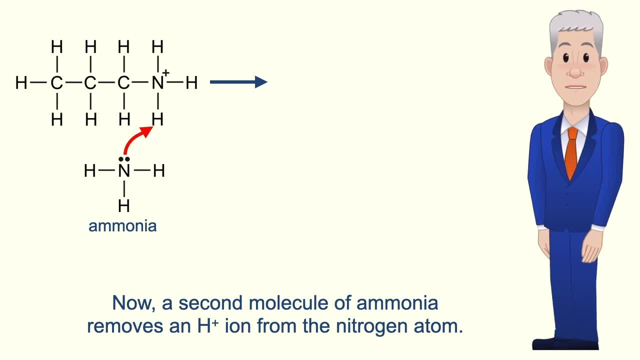 ion. Now a second molecule of ammonia removes an H-plus ion from the nitrogen atom. The covalent bond between the hydrogen and nitrogen breaks, with both electrons moving onto the nitrogen. At the end of this stage we've made the product 1-aminopropane, which is a 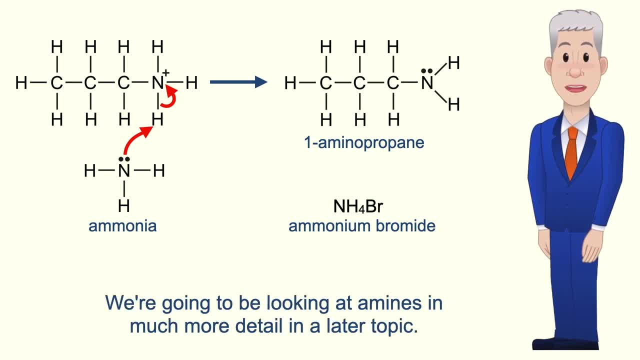 primary amine. We're going to be looking at amines in much more detail in a later topic. We've also made the ammonium ion NH4+- The ammonium ion and bromide ion form ammonium bromide. Now, to carry out this reaction, we warm our haloalkane with a concentrated ammonia solution in ethanol. 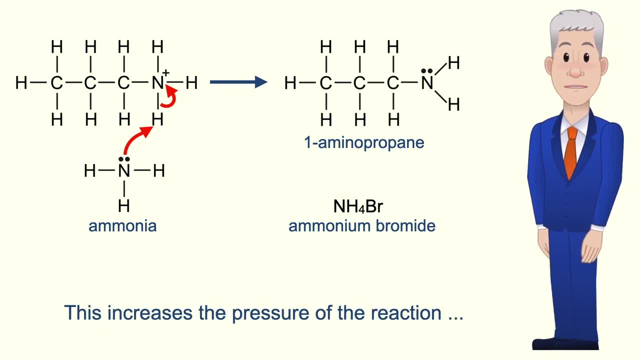 This reaction is carried out in a sealed tube. This increases the pressure of the reaction and prevents the ammonia escaping as a gas. Also, it's important that we use an excess of ammonia. As you can see in the product amine, the nitrogen atom still has a lone pair of electrons, so this can also act as